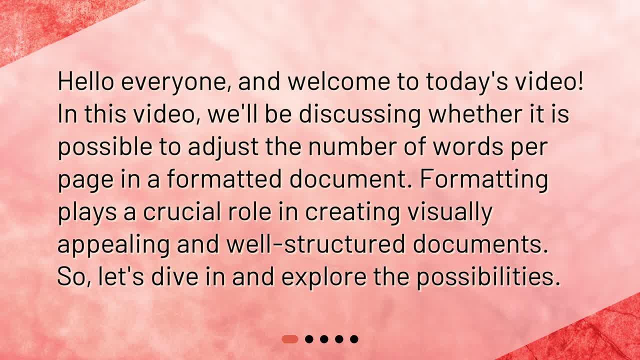 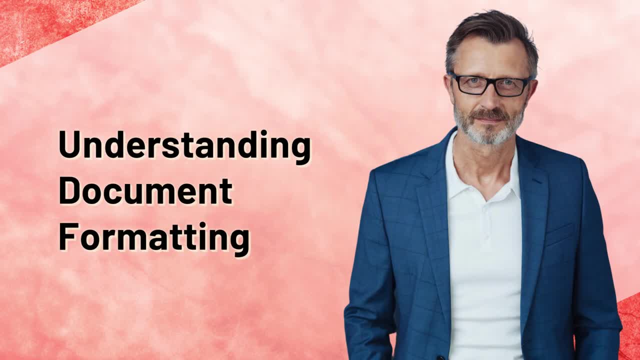 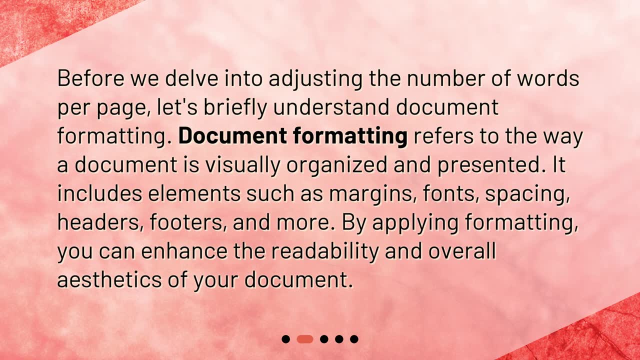 role in creating visually appealing and well-structured documents. So let's dive in and explore the possibilities Understanding Document Formatting. Before we delve into adjusting the number of words per page, let's briefly understand document formatting. Document formatting refers to the way a document is visually organized and 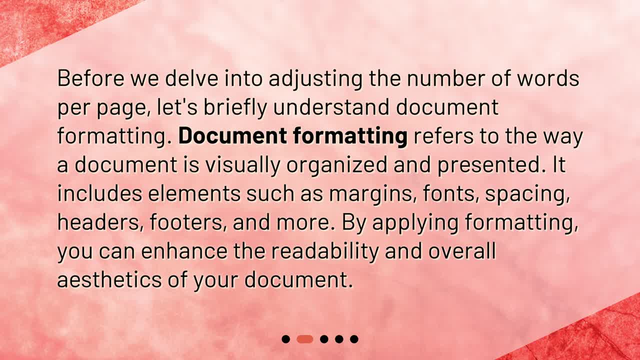 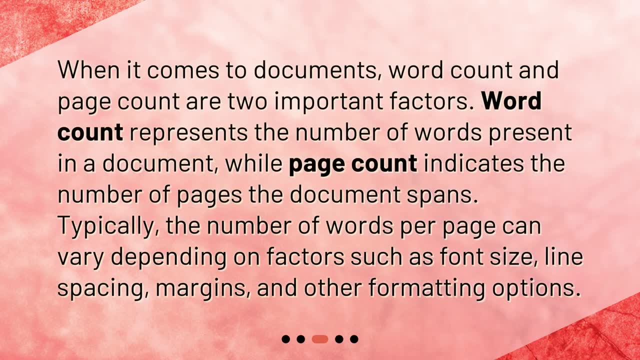 presented. It includes elements such as margins, fonts, spacing, headers, footers and more, Word Count and Pages. When it comes to documents, word count and page count are two important factors. Word count represents the number of words present in a document. 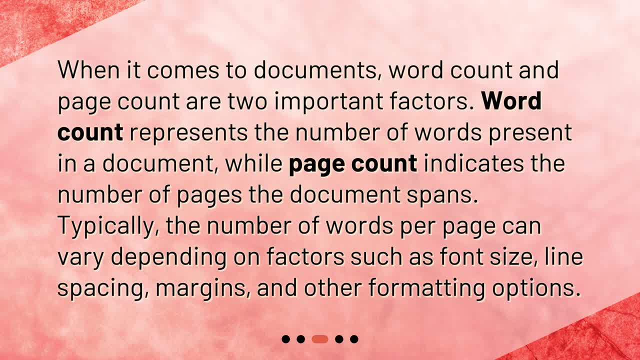 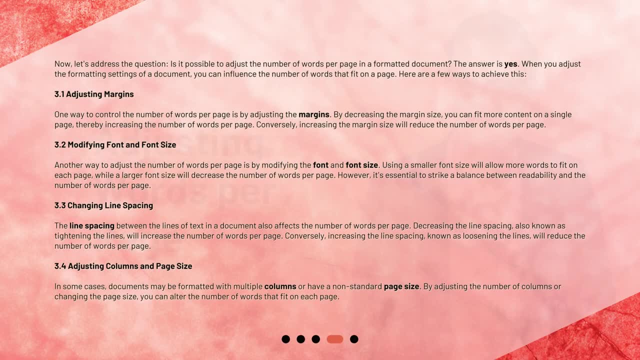 while page count indicates the number of pages the document spans. Typically, the number of words per page can vary depending on factors such as font size, line spacing, margins and other formatting options. Now let's address the question: Is it possible to adjust the number of words per page in a 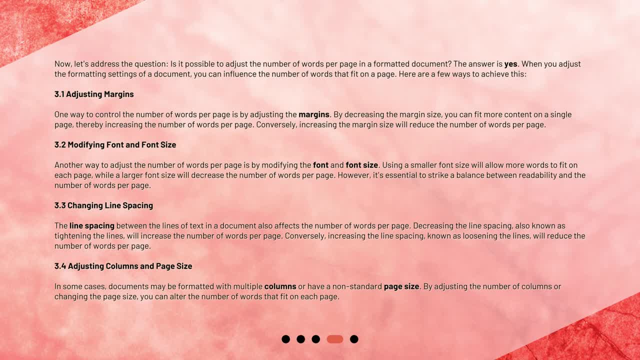 formatted document. The answer is yes. When you adjust the formatting settings of a document, you can influence the number of words that fit on a page. Here are a few ways to achieve this. 3.1: Adjusting Margins. One way to control the number of words per page is by adjusting the margins. 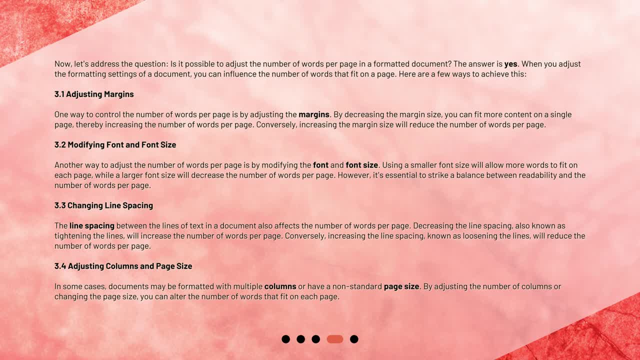 By decreasing the margin size, you can fit more content on a single page, thereby increasing the number of words per page. Conversely, increasing the margin size will reduce the number of words per page. 3.2: Modifying Font and Font Size. Another way to adjust the number of words per page is by modifying the font and font size. 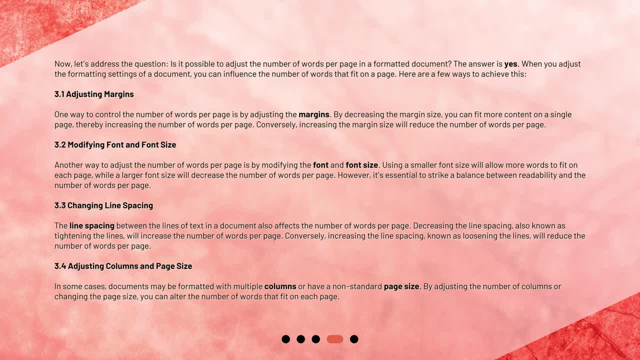 Using a smaller font size will allow more words to fit on each page, while a larger font size will decrease the number of words per page. However, it's essential to strike a balance between readability and the number of words per page. 3.3: Changing Line Spacing. 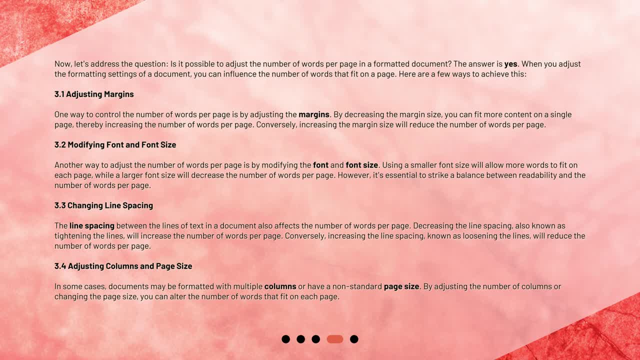 The line spacing between the lines of text in a document also affects the number of words per page. Decreasing the line spacing, also known as tightening the lines, will increase the number of words per page. Conversely, increasing the line spacing, known as loosening the lines.